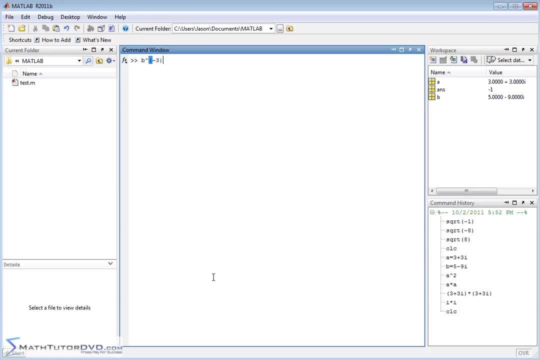 do things like raise things to a negative power. So this b to the negative 3 would be- and b, by the way, is given, we've already defined it- 5 minus 9i. So when you raise it to a negative power, it's like saying 1 over b cubed And it does all that math for. 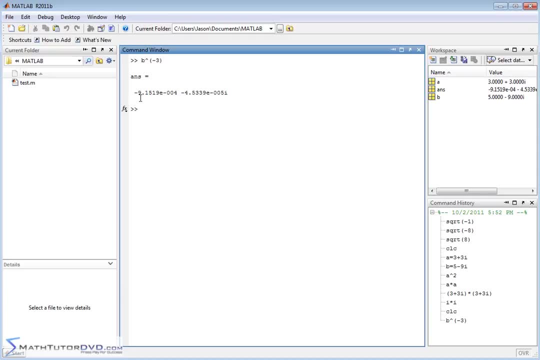 us, And so we have a very small real part negative 9.15 times 10 to the negative 4.. The imaginary part is also very small, So we have a very small real part negative 9.15 times 10 to the negative 5.. So it does all that stuff behind the scenes, which is great. 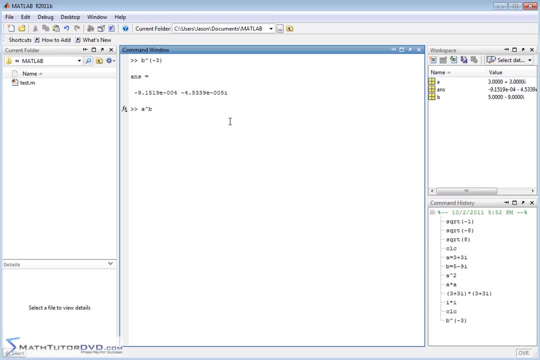 We can actually do things like taking a complex number and raising it to another complex number, because a and b are both complex, And when you do that, MATLAB does all the heavy lifting and computes the answer, So it behaves much like a calculator. You might expect a high-end. 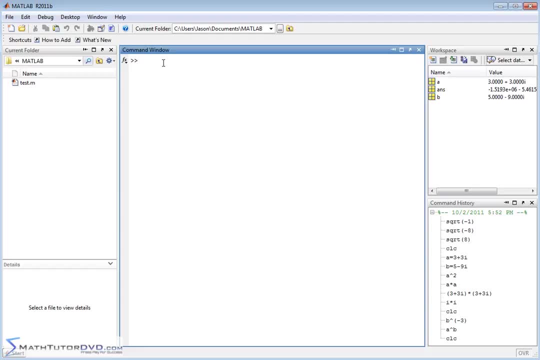 calculator to do Now. another thing is there are a lot of built-in functions in MATLAB. There are a lot of functions that are specifically designed to basically operate on complex numbers. One of them is the absolute value. The absolute value, as you know from basic algebra of 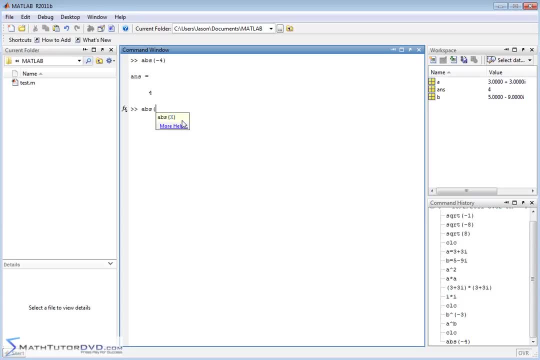 negative. 4 is just 4, right. But this absolute value function also works just fine on complex numbers. So this is a complex number. a is 3 plus 3i, So what it's going to do is calculate the magnitude of this guy and it will always respond with a positive number. So what's going on here? if you look into the, 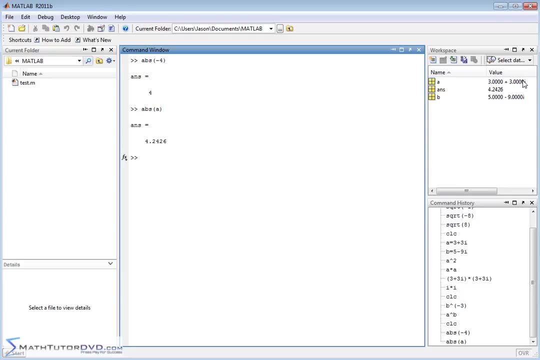 math behind it is: you're doing the Pythagorean theorem on the real part and the imaginary part and you're getting the answer, and that's what we call the absolute value or the magnitude of that complex number. Now, this complex number lies in the complex plan as well. You have a real part and an imaginary part. 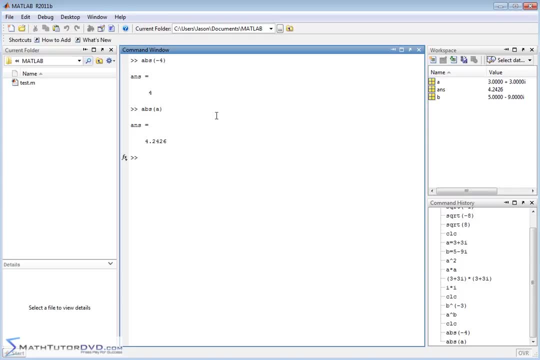 So there's always an angle defined with every complex number: the angle from where you are to the x-axis. So to pull that angle out, you just basically type in angle and then you pass it the complex number and it's going to respond. 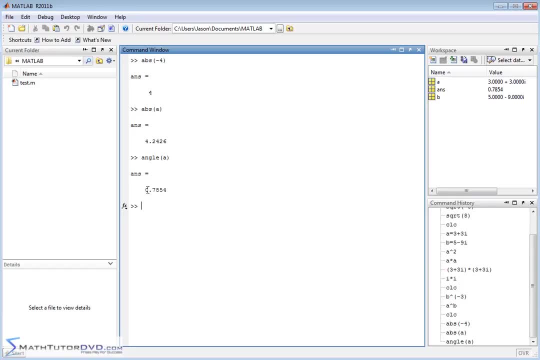 Now you should know by now, MATLAB always deals in radians, so this is an angle in radians. If you wanted that to be in degrees, you would say: okay, let's take what we did before. Take the angle of that complex number. We need to multiply it by 180, divided by pi. 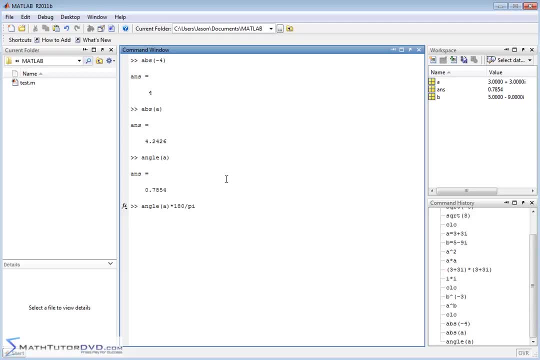 That's going to cancel radians with radians, and so you're going to be left with degrees. That's just a conversion factor. so that's 45 degrees And that should make sense to you, because the complex number a is 3 plus 3i. 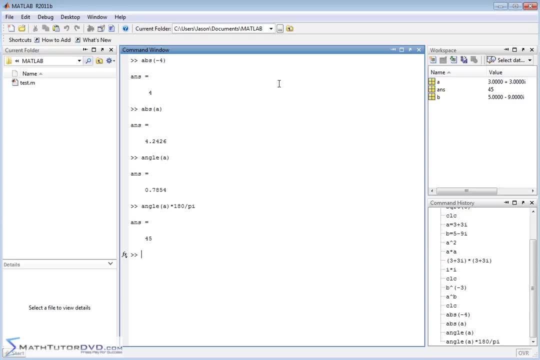 So it's 3 units over on the real axis, 3 units up the imaginary axis. It should be right at 45 degrees and that's what we get. So doing the absolute value of a complex number and the angle that exists in the complex number. 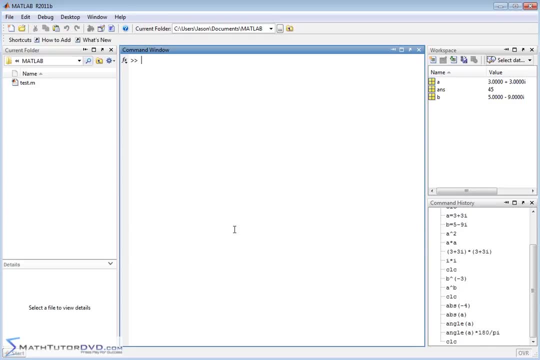 is something you'll be doing a lot with any time you deal with any kind of complex results. The other thing is, I just want to show you that this absolute value business makes intuitive sense if you just operate on pure imaginary numbers. There's no real part to this at all. 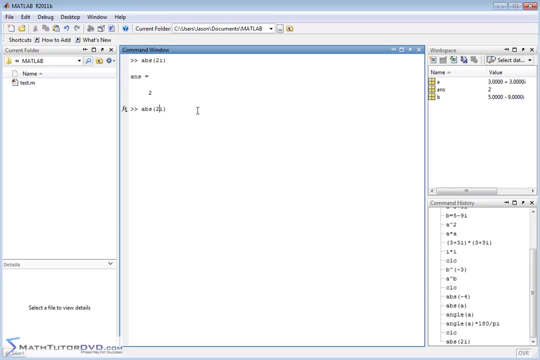 So the absolute value should be 2.. If you have 3i, the absolute value should be 3, and so on. So if you pass it- a complex number- to plus 3i, then, like I said before, it's doing the Pythagorean theorem to find out what the magnitude there is. 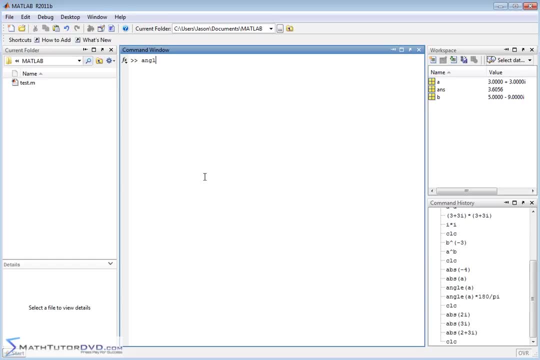 Same thing for the angle. just to kind of review a little bit. If you have a pure imaginary number, see, this is a pure imaginary number, There's no real part to it, It's just imaginary. So the real part is 0.. 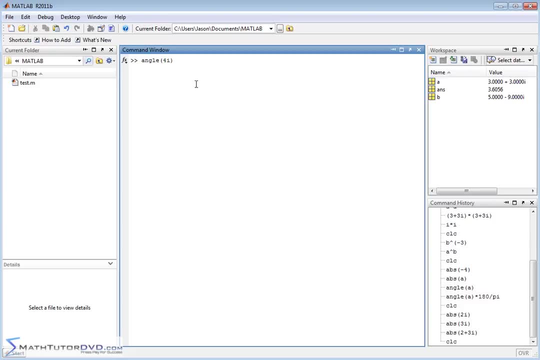 The imaginary part is straight up and down on the imaginary axis, So the angle for something like this is always going to be 90 degrees, or pi over 2.. This is pi over 2 radians, And if you didn't believe me there, you could just multiply by 180 over pi. 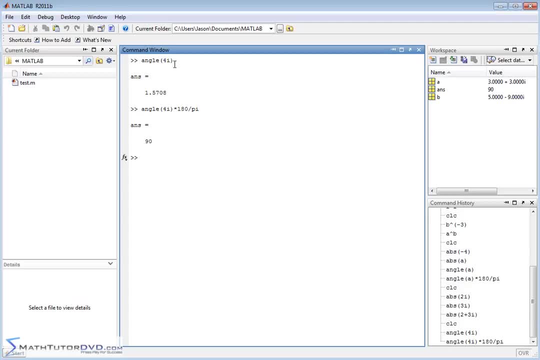 which is our conversion factor and that's 90 degrees. So any kind of pure imaginary number when you're trying to find the angle is going to give you that. So whenever you do something like angle B, which is over here, we have 5 minus 9i. 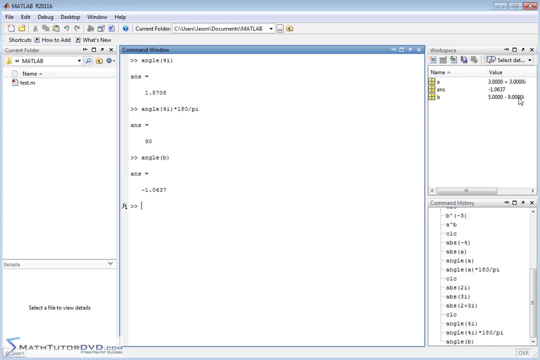 then what you're doing is you're basically taking the inverse tangent of this divided by this- That's all given in your math books- to find that angle. In this case it's negative, blah, blah, blah radians. And you can multiply by 180 divided by pi to give you the angle in degrees. 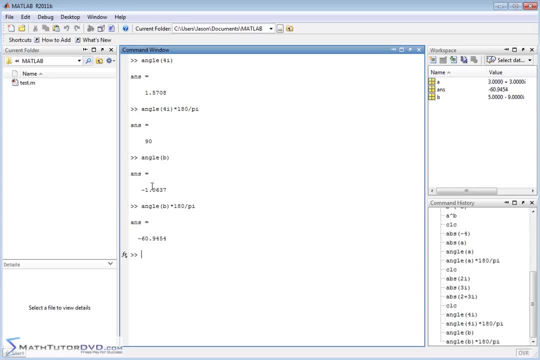 So it's almost negative. 61 degrees would be the angle where that complex number lies. All of this stuff is taught to you when you start learning about complex numbers. I'm just kind of going through some real calculations so you can kind of get familiar with how you deal with it in MATLAB. 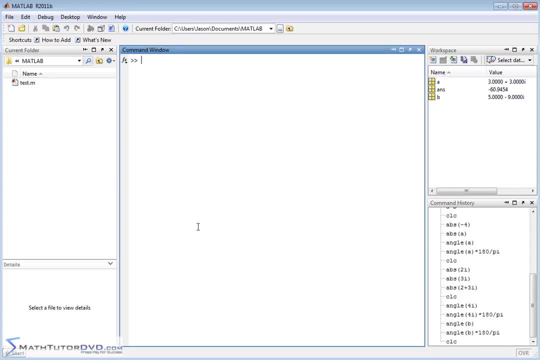 Now you also have some other functions that are designed specifically to deal with complex numbers. For instance, there's a function called real, And if you pass it something like this, then it's going to return. whatever the real part of this is, 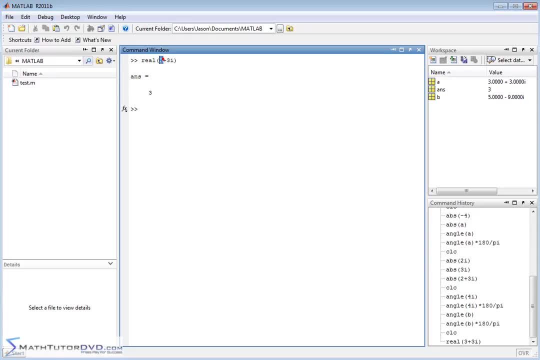 So this is the real part, This is the imaginary part, so it's going to return 3.. Of course, it's perfectly happy if you put a variable in there that has a complex number: Right, 5 minus 9i. 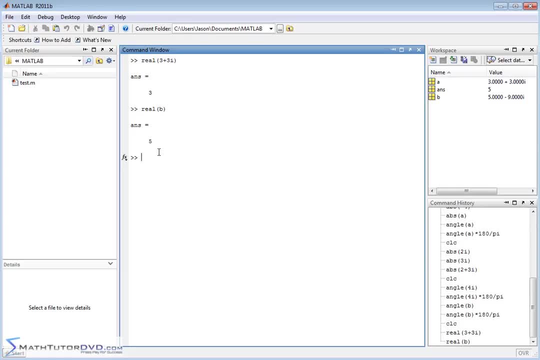 That's what I'm putting in there, So the real part of that is 5.. So it's just going to return this guy. The same thing works just fine with imaginary. If I stick the variable a into the function called imaginary- i, m, a, g- then this variable is going to go in there. 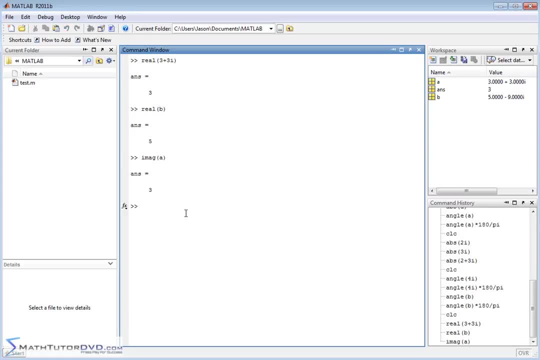 The imaginary part is 3.. So the imaginary part is going to return 3.. If I stick variable b in there, if you look at what b is, the imaginary part is negative 9.. So it's going to return with negative 9.. 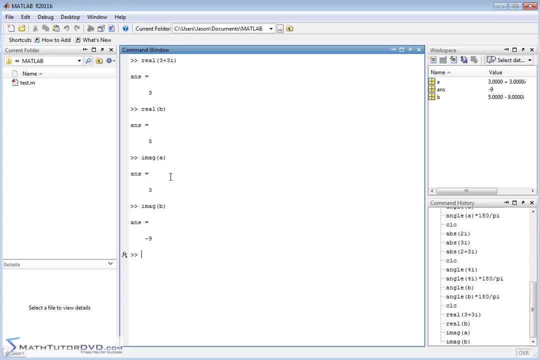 These are things that really are not something you can do. You would probably not do them so much when you're just working with these basic complex numbers, But you might use them a lot if you're programming in MATLAB. Maybe you're writing a function that you've got a very long calculus, integration or something like that that you're doing. 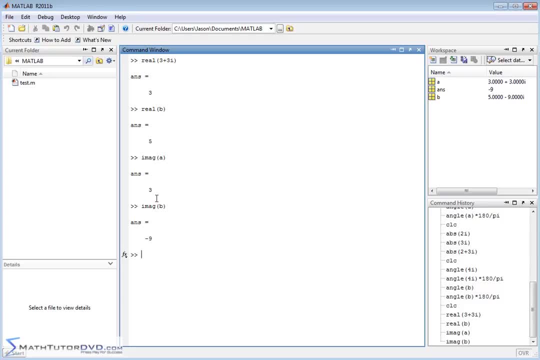 the result of which might be complex. Well then, your final answer. maybe you want to strip away the imaginary part and only give yourself the real part. in the final display of the answer, Let's just say: whatever integral you're doing, you only care about the real part of the result. 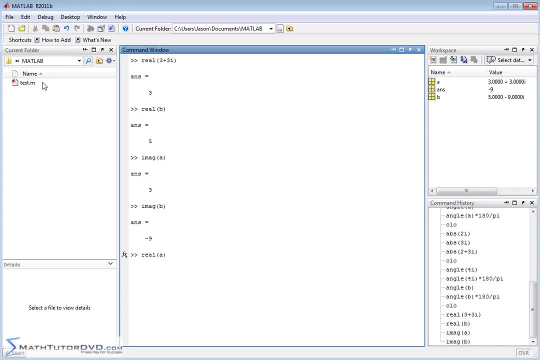 So you might have a function in one of these m files that calculates the integral. it gets a complex answer and then you might, at the very end, just take the real part of it and display the real part as the answer. Maybe that's just your algorithm. 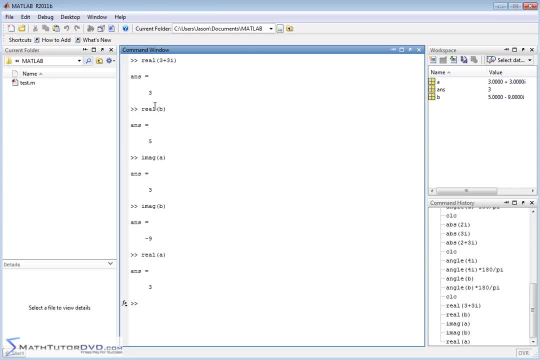 So these functions- real and imaginary, absolute value, angle, things like that. those are things that are kind of trivial, but you might use them when you're programming, So that's why we're really covering them. Okay, let me clear the screen. 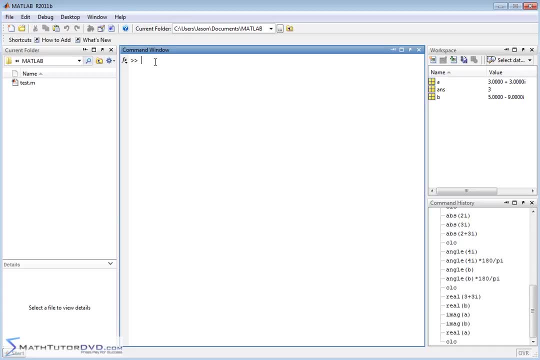 Finally, before I close here, I'd like to just kind of go over some things, Something very important with complex numbers that you learn in your math classes, in trigonometry and in calculus in specific. So, if you remember, there's something called the Euler identity right. 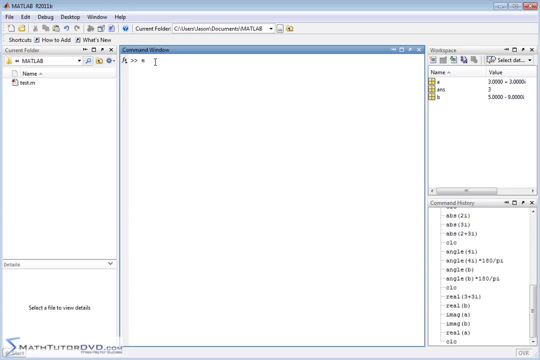 And that means that if you have a complex exponential right, For instance, something like pi times i, okay, So this is a complex exponential. In other words, it's e raised to the power of pi times i. And if you have learned about the Euler identity, 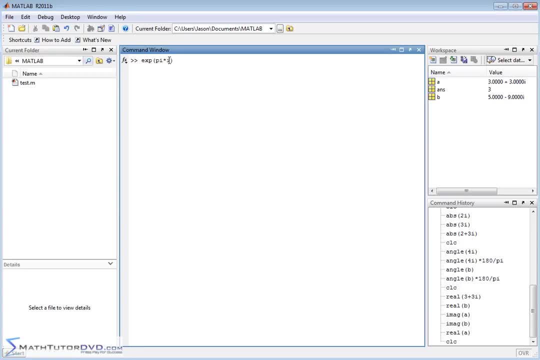 which most of you probably have, then what it means is that this is an equivalent way of writing a complex number. The magnitude of this guy- remember the absolute value we're just calculating- is whatever sits out in front of this exponential, which, in this case, is 1.. 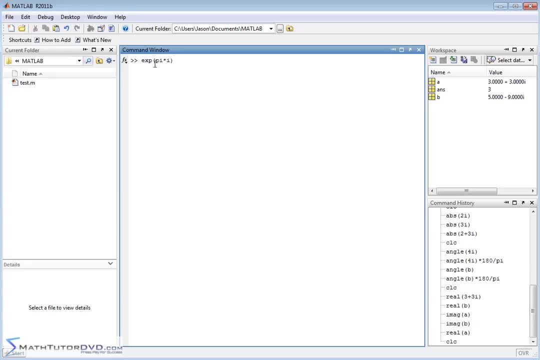 The angle, which, remember we were using the angle function, is basically the angle here that sits in front of the i. So I can just look at this without doing any calculations and I can see that the magnitude, the absolute value of this complex number. 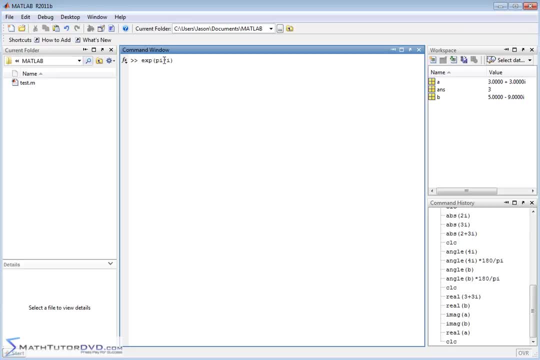 is 1, and the angle is pi, And that's just because of the way it's written here. Now, whenever you deal with complex exponentials, sometimes you want to convert them back and forth from polar form like this or, I guess, complex exponential form. 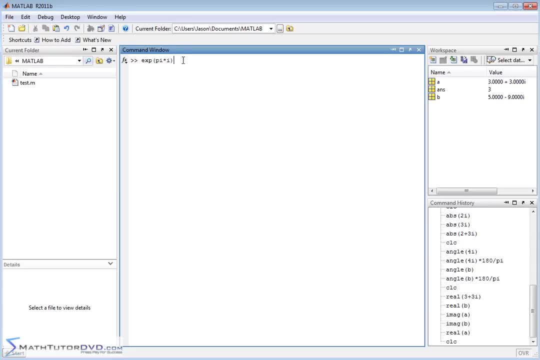 you might want to convert them to rectangular form. So when you type it in like this and you hit enter, MATLAB is going to basically automatically convert it to rectangular form. So MATLAB says that from the Euler identity, from the math behind it, this is equivalent to negative 1 plus 0i. 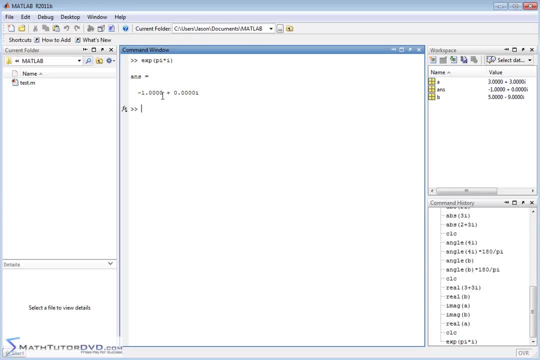 In other words, it's equivalent to saying the real part's negative 1, the imaginary part is just 0. And so that comes about because the Euler identity is cosine of the angle, plus i times the sine of the angle. The angle here is pi. 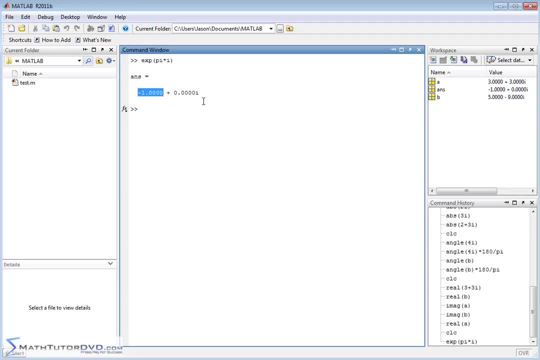 So cosine of pi is negative 1,. okay, that's the real part plus i times the sine of this angle and the sine of pi is 0i. So that's cosine plus i sine of the angle and that is the Euler identity and that's why you get this. 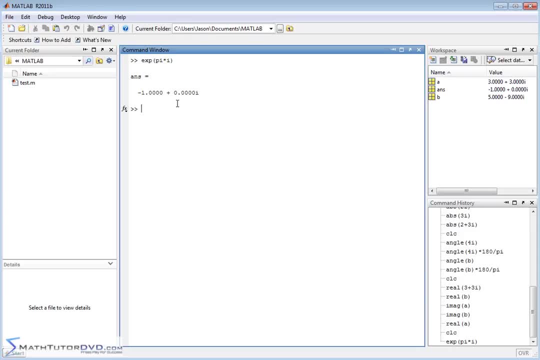 Now, if you were to just take the absolute value of exponential pi times i, and so basically this e to the pi i, you wrap it inside of the absolute value function, what you should get is the absolute value of this complex number which we already said, the absolute value. 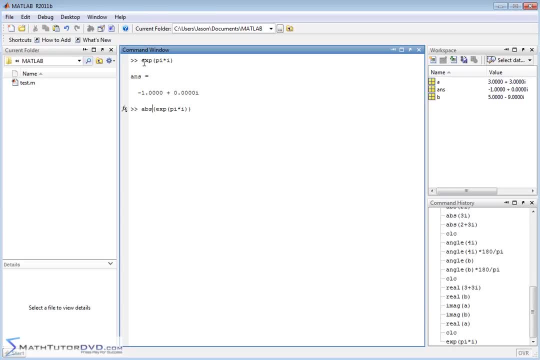 when you write it like this, you learn from your math is just whatever sits out in front of the exponential, which is 1.. So the absolute value, which is the magnitude of this complex number, is 1.. So let me go back and change the function. 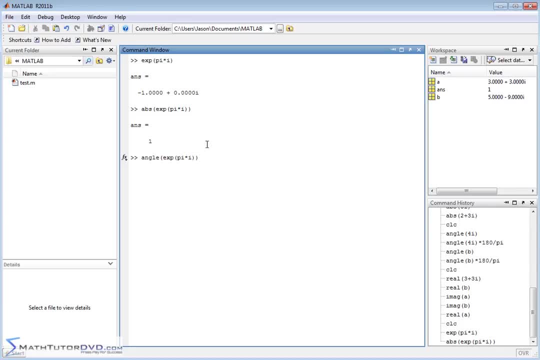 Instead of absolute value. what if we type in angle? What we're trying to find here is: what is the angle that this complex number sits at? Well, the magnitude's what sits in front of the exponential. The angle here is the angle in radians that we have. 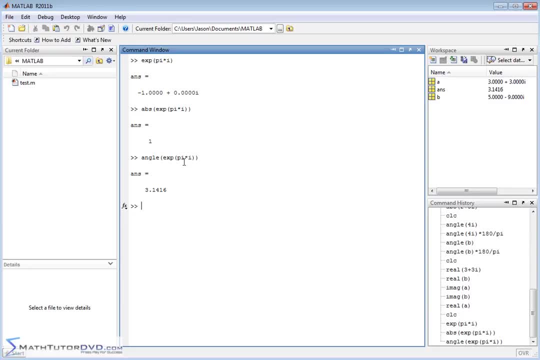 So if you hit this guy, then what you're going to get is 3.14, that's pi. So I'm just telling you in a roundabout way that MATLAB understands this. It understands Euler's identity, It understands all of the identities, basically. 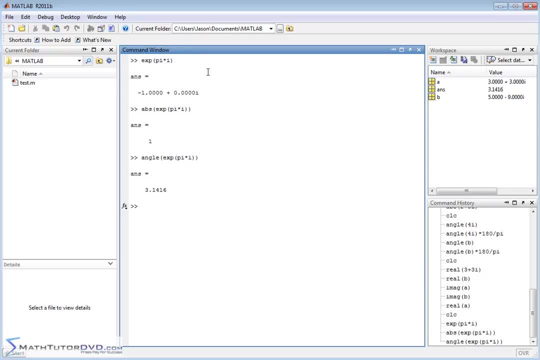 So if you type a complex exponential in, MATLAB's going to convert it to rectangular for you. If, for some reason, you would like to extract the magnitude and the angle, it totally understands. if you put them in complex exponential form, it'll give you the absolute value, it'll give you the angle back. 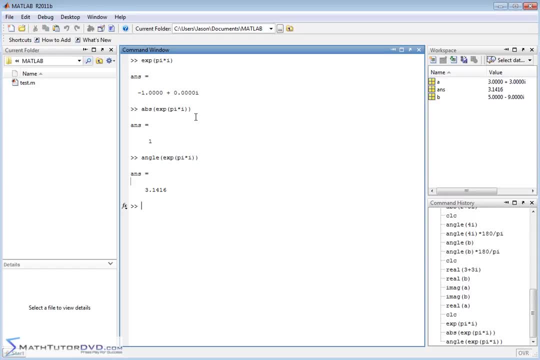 Or, like we did in the last section, if you put these guys in rectangular form, like we did in the last section, it understands how to calculate the absolute value and the angle. So sort of the bottom line to take away from this is MATLAB completely understands. 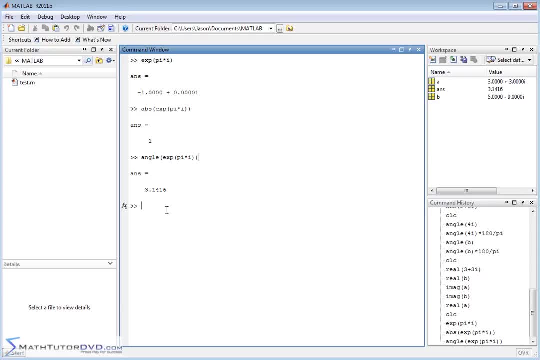 no matter how you enter your complex number, how these functions that operate, that return, magnitude and angle, it understands how to do all the calculations behind the scenes. One final example: Let's say that, for instance, I want to take the absolute value of the complex number.